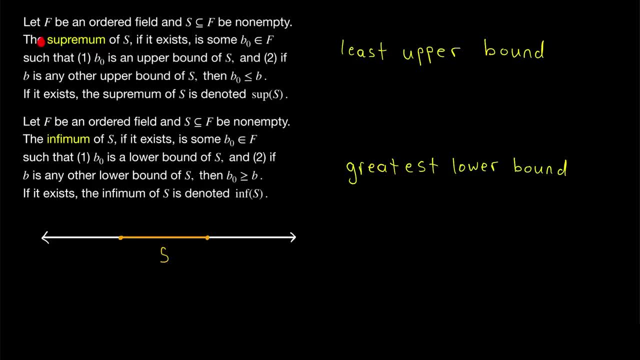 the ordered field that we're most interested in, Then the supremum of S, that non-empty subset of the ordered field, the supremum of S, if it exists, is some B0 from the ordered field, such that 1 is an upper bound of S and 2, if B is any other upper bound of S, then B0, the supremum is less. 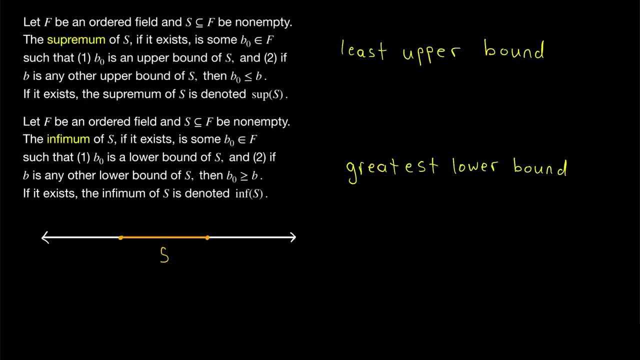 than or equal to B that other upper bound. That should make sense, because the supremum is the least upper bound. So if B0 is the supremum and B is any other upper bound, B0 must be less than or equal to that other upper bound B. If the supremum of S exists, it's denoted like this: 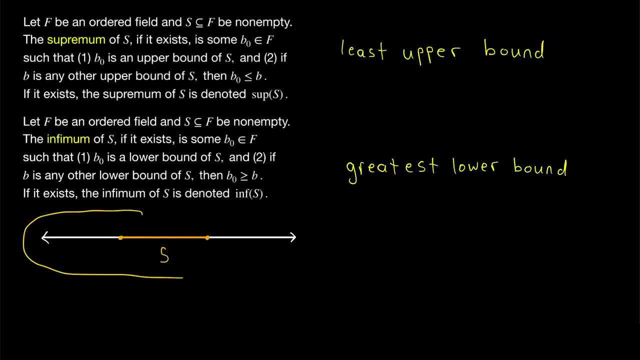 of S For visual representation of what we're talking about. suppose this down here is the real number line and maybe this orange part S, is a subset of the real numbers, Then certainly this number here is an upper bound of S. Every element of S is less than or equal to this number up here. 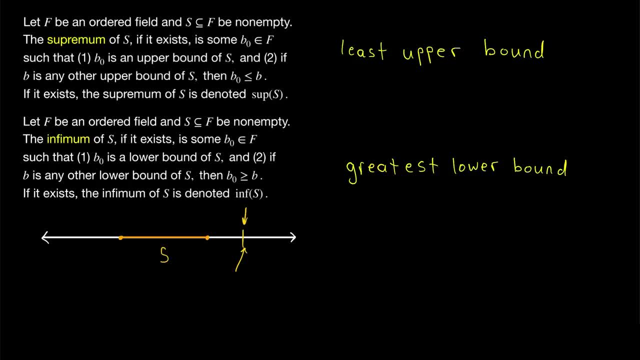 However, it's not the least upper bound, so it's not the supremum. There are upper bounds, much less than this one represented by this orange part, so it's not the supremum. We could get a lot closer to S, say right there. That is what the least upper bound might look like. 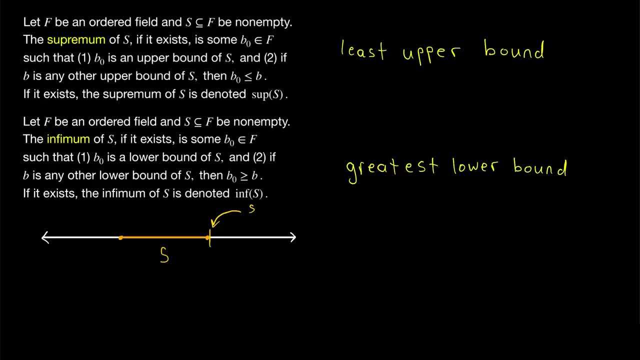 visually, and so that is a representation of the supremum, of S, the least upper bound. We've got all these other upper bounds up here, but that's the smallest one. Alright, now for the infimum. Let F be an ordered field and S be a non-empty subset. 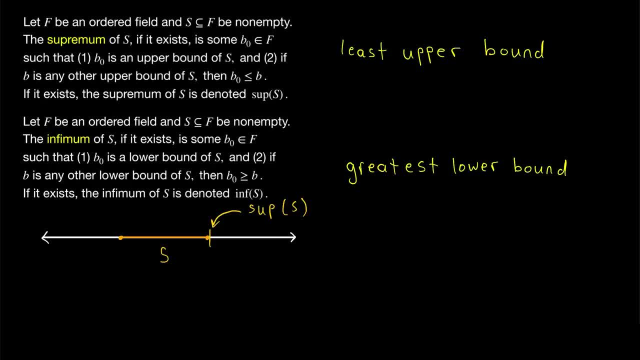 of that ordered field. Again, you can just think of S as the real numbers if you want. The infimum of S, if it exists, is some B0 from the ordered field or from the real numbers. that satisfies two conditions. One, B0 is a lower bound of S and two, if B is any other lower bound. 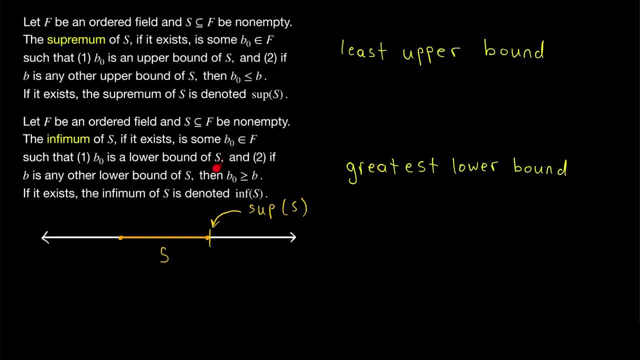 of S, then B0, the infimum is greater than or equal to that other lower bound, B. Again, that should make sense, because B, the infimum, is the greatest lower bound. So if we've got any other infimum of S, then the infimum, B0, must be greater than or equal to that other lower bound. 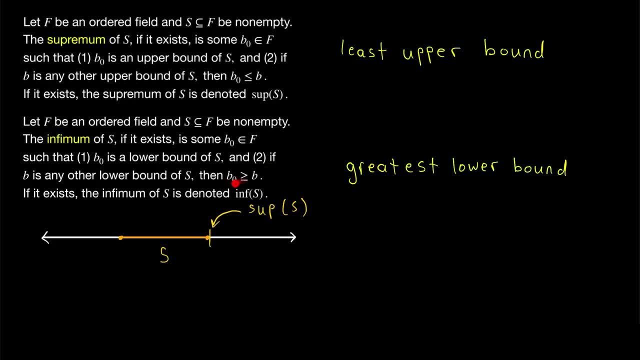 So if the infimum of S exists, it's denoted like that inf of S. Let's again represent that visually with this number line: Certainly, this number back here is a lower bound of the set S. Every element of S is greater than or equal to this number back here. 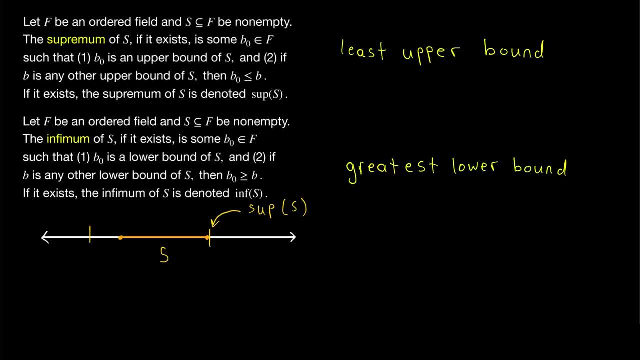 However, it's not the greatest lower bound, so it's not the infimum of S. The greatest lower bound would look something like that: Of all lower bounds, this is the greatest one, and so visually that's a representation of the infimum of S. Notice, these definitions don't. 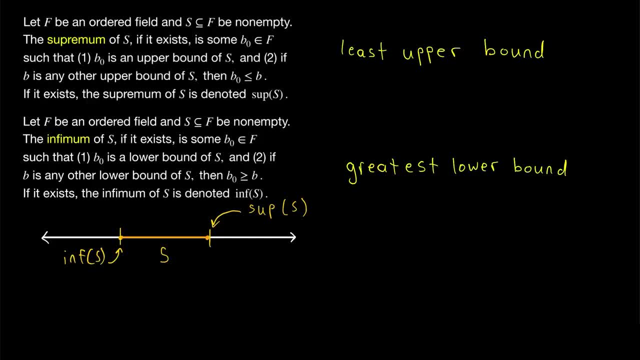 explicitly state the supremum and infimum of a set are unique, but it turns out they are, and I'll leave a link to a proof of that in the description. Remember these three-word descriptions and you should be good to go. The supremum of a set, if it exists, is the least of. all of them. So if you have a set that exists, it's the least of all of them. So if you have a set that exists, it's the least of all of them. So if you have a set that exists, it's the least of all of them. 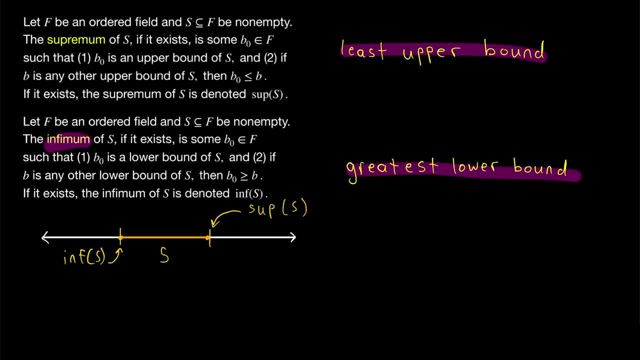 The supremum of a set, if it exists, is the greatest of all lower bounds. The infimum of a set, if it exists, is the greatest of all lower bounds. One last thing to point out before we move on. note that both the infimum and supremum, they do not have to belong to the set S, They just have. 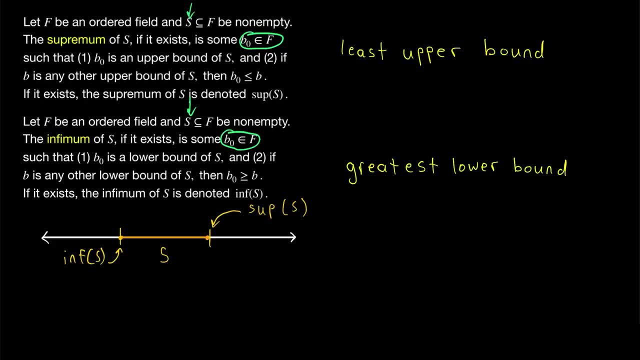 to belong to that ordered field F. that S is a subset of. So the supremum and infimum of a set may or may not actually belong to the set. There are examples of both. Additionally, we could consider a set of the set S as a subset of the set S. So if you have a set S you could consider. 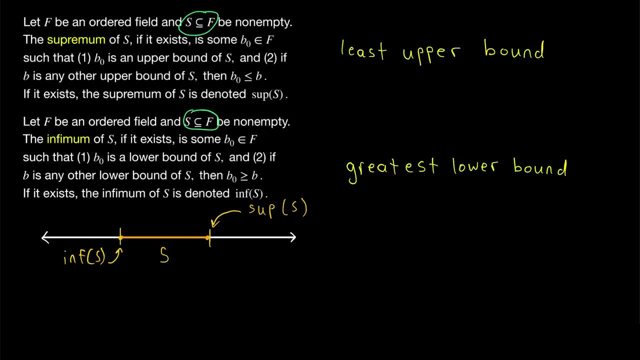 a set to be a subset of many other sets. For example, the natural numbers are a subset of the integers. However, the natural numbers are also a subset of the real numbers, So the ordered field under consideration in a given problem can change whether or not the subset S will or will. 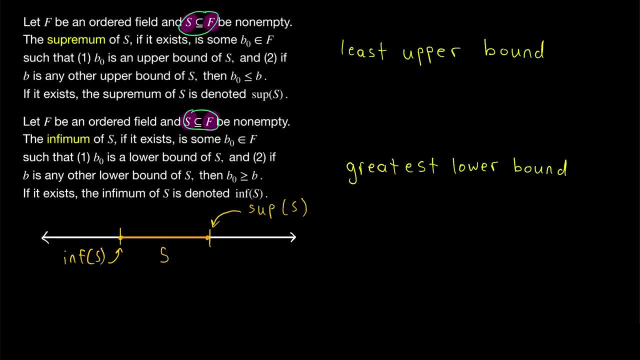 not have a supremum and infimum. That's an important technicality of the definition. but of course, for many of you the ordered field you're considering will probably be the real numbers. But let's get into the examples and we'll see an instance of where the ordered field chosen does matter right. 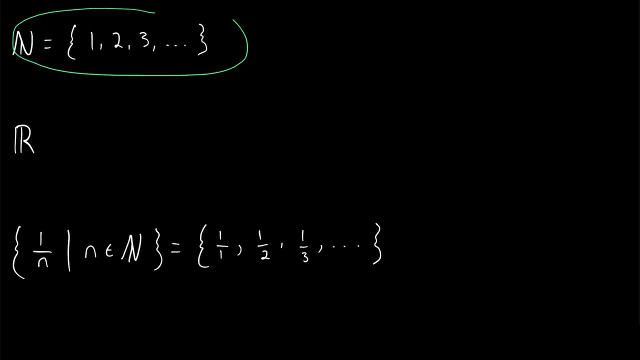 near the end. All right, let's get into it. Here is the set of natural numbers. Does this set have a supremum? Well, no, it doesn't, Because, remember, the supremum is the least upper bound if it exists. The natural numbers have no upper bound. You could give me any natural number, say 10 to the power of 10, and I could give you any natural number, say 10 to the power of 10,. and I could give you any natural number, say 10 to the power of 10, and I could give you any natural number, say 10 to. 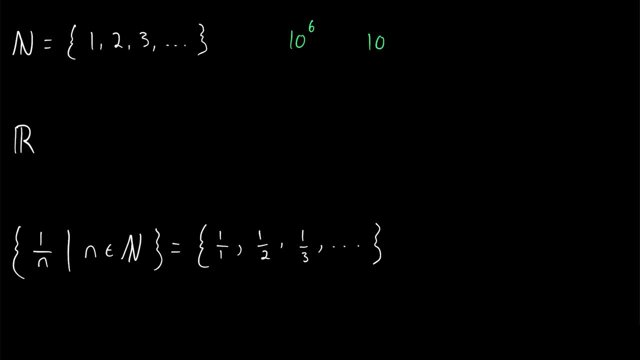 the power of 6, and I could guarantee you that's not an upper bound of the naturals, because 10 to the 6 plus 1 is also a bigger natural number. So the supremum of the naturals does not exist. What about the infimum? Remember that the infimum is the greatest lower bound. Certainly, 0 is a 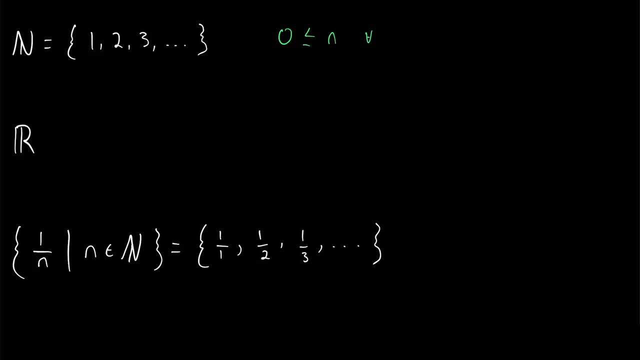 lower bound of the naturals, 0 is less than or equal to n for every n in the natural numbers. However, 0 is not the infimum of the natural numbers because it's not the greatest lower bound. 1 is also a lower bound of the naturals because it is less than or equal. 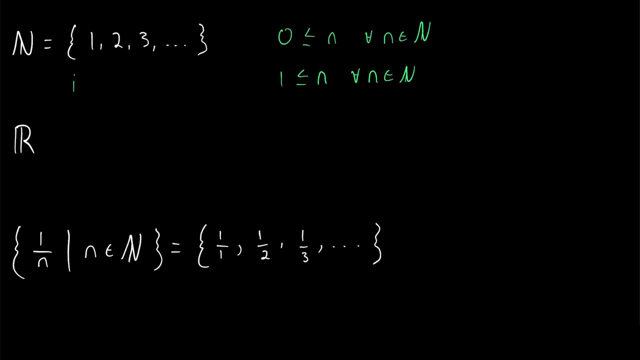 to n for every n in the naturals too, And so we can certainly include that the infimum of the natural numbers, inf of the naturals, is equal to 1.. Any number bigger than 1 would not be a lower bound of the naturals, because 1 would be less than it. So certainly the infimum of the naturals is 1.. 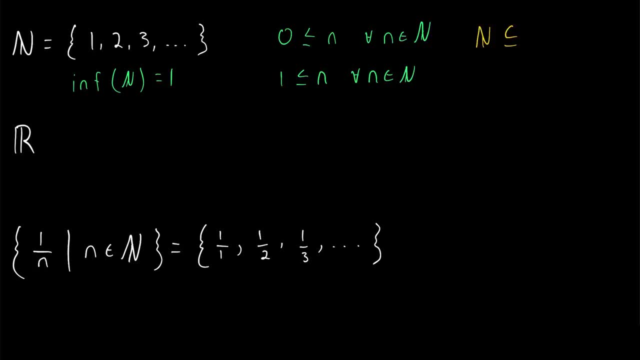 And note. for this example, it doesn't matter whether we're considering the naturals to be a subset of the ordered field of rationals or if we're considering the naturals to be a subset of the ordered field of real numbers. Either way, it doesn't have a supremum and it does. 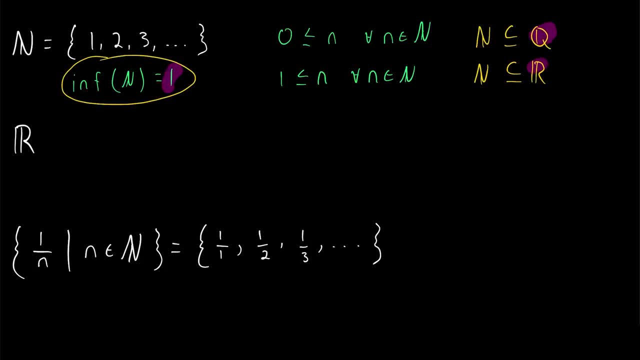 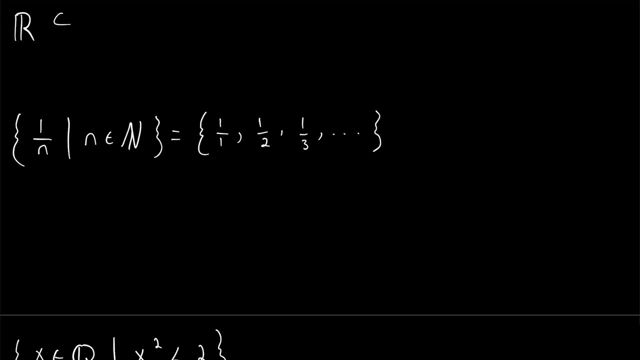 have an infimum. 1 is both a rational number and a real number, so we're good to go either way, All right. next example: How about the real numbers? Of course, the real numbers are a subset of themselves, so we might consider the real numbers to be the subset and the 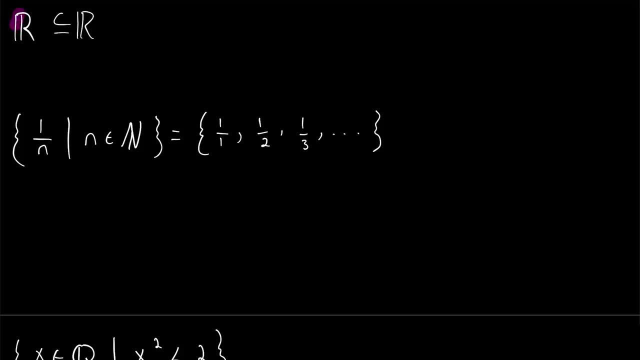 broader ordered field under consideration here, But certainly neither the infimum nor the supremum of the real numbers exists. The infimum is the greatest lower bound. The real numbers have no lower bound. The supremum is the least upper bound. The real numbers have no upper bound. 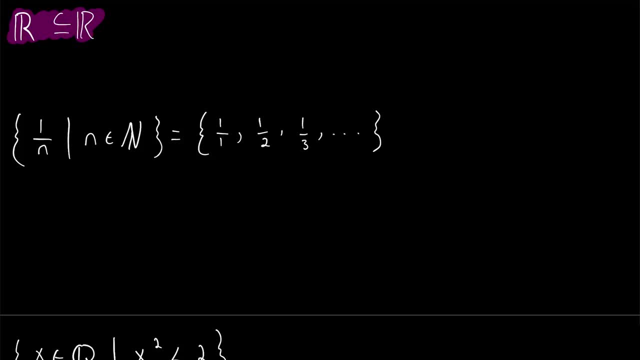 The reals are an unbounded set below and above, so the reals have no infimum and no supremum. All right. second to last example, Got some set builder notation going on here. This is a set of all numbers 1 over n, where n is a natural. The set looks something like this: 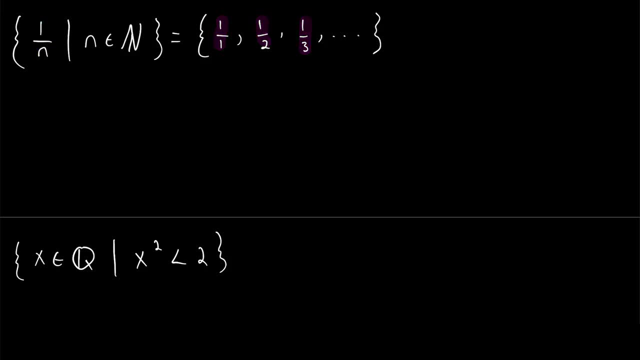 1 over 1, 1 over 2,, 1 over 3, and so on. You may quickly notice that the biggest number in this set is 1 over 1, which is just 1.. The numbers just keep getting smaller after that, So 1 is an upper bound. 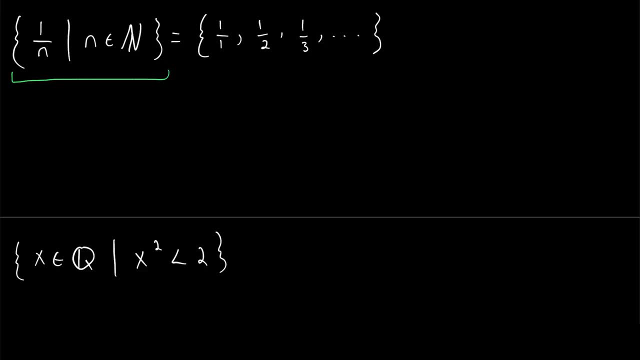 of this set? Is it the least upper bound? Is it the supremum? Yes, it certainly is. If we consider any number smaller than 1, it wouldn't be a set of all numbers, 1 over n, where n is a natural. 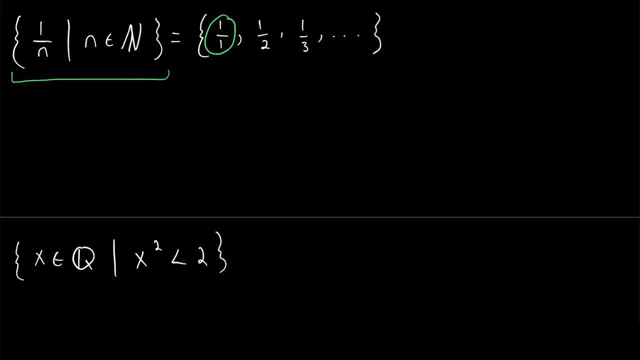 It wouldn't be an upper bound because 1 is in the set, So you can't get an upper bound smaller than 1.. So 1 is the least upper bound, Thus the supremum sup of this set. I'll just paste it into: 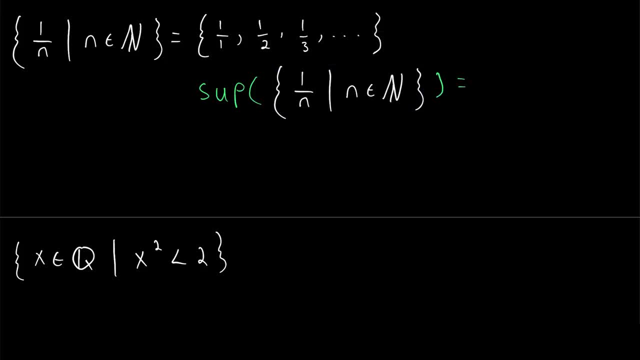 our sup function sup of this set is equal to 1.. It is the least upper bound. All right, now how about the infimum of this set? Does the infimum exist? Well, certainly the elements of this set are just getting smaller and smaller for larger values. So 1 over n is the least upper bound. 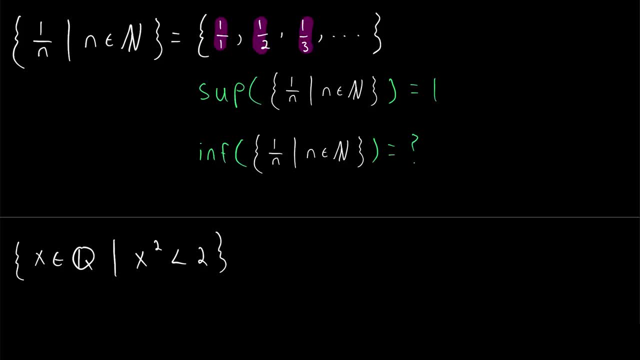 However, they never get negative. In fact, what they do is get closer and closer to 0.. We know that 0 is a lower bound of this set, because 0 is less than or equal to the reciprocal of every natural number. And certainly, if we consider any number, say epsilon, greater than 0, we would be 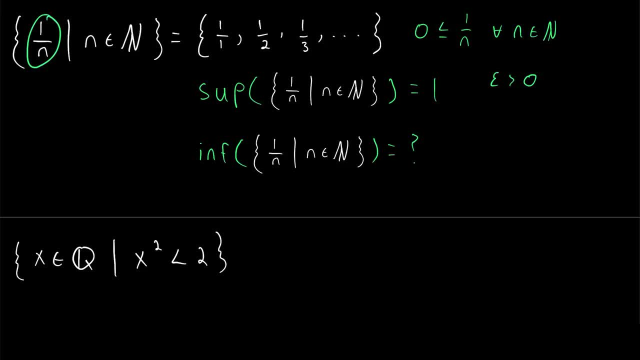 able to find an n big enough so that 1 over n is less than epsilon, And thus epsilon would be a lower bound. So of all lower bounds, 0 is certainly the greatest one and is thus the infimum. So the infimum of this set is 0.. And don't worry if you didn't understand that fully, I'm not. 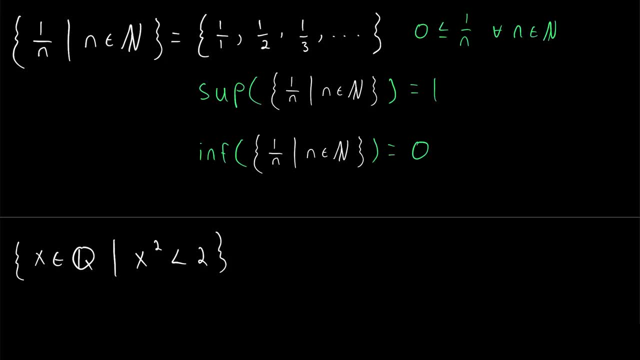 trying to give you rigorous proofs of these results. just rough explanations, And we'll go over some more rigorous proofs of this sort of thing in future lessons. It's just important that you have a feel for why 0 is the infimum of this set. Notice in this example that 0 is the 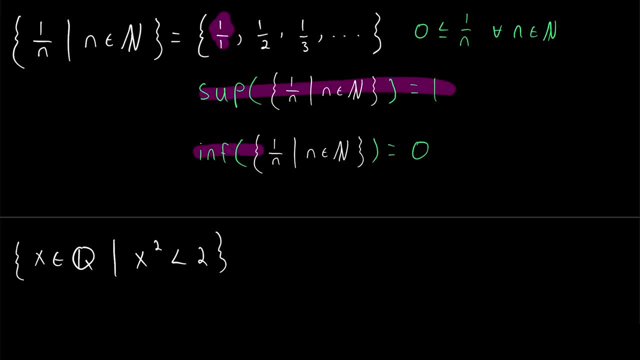 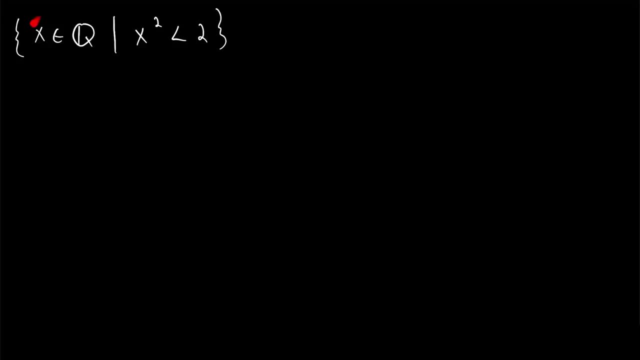 the supremum of the set is in the set, whereas the infimum of the set is not in the set. All right, now we've got our last, most interesting example. This is the set of all rational numbers whose square is less than 2.. And for now, let's consider this set to be a subset. 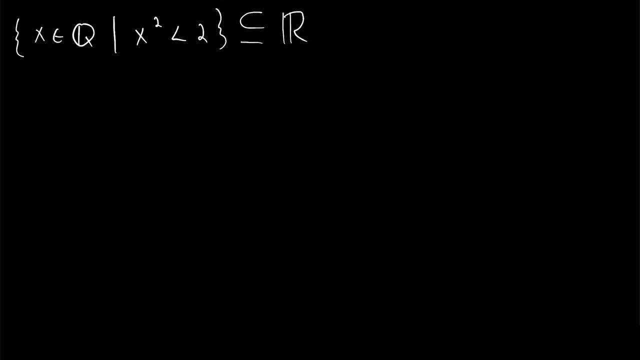 taken from the ordered field of the real numbers, We know that all elements x from this set satisfy this inequality. Their square x squared is less than 2.. This means that the absolute value of x has to be less than the square root of 2.. Remember that. 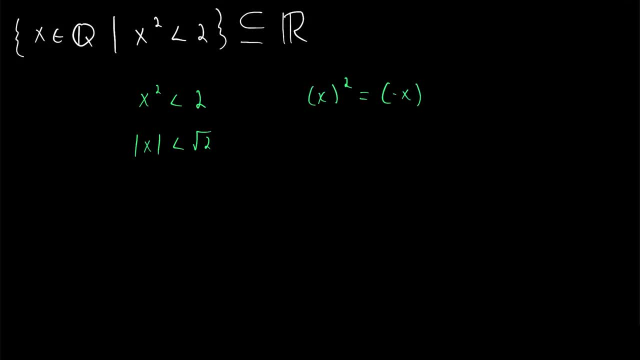 x squared and negative x squared are both equal to x squared, which is why we have to involve the absolute value bars here. In a previous lesson, which I'll leave a link to in the description, we showed that an inequality like this implies the following: that x must be less than the square. 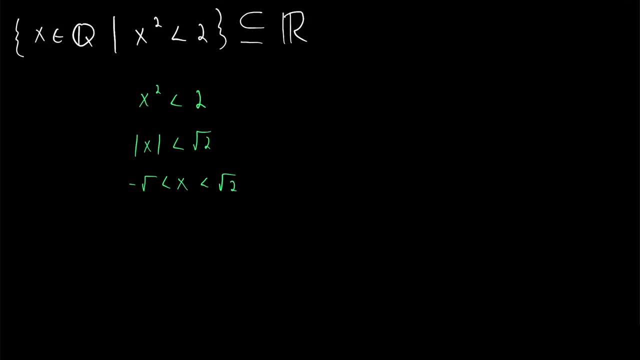 root of 2 and must be greater than x squared. And so in this example we have a set of all negative square root of 2.. So, clearly, negative square root of 2 is a lower bound on the elements of our set, and positive square root of 2 is an upper bound on the elements of our set. 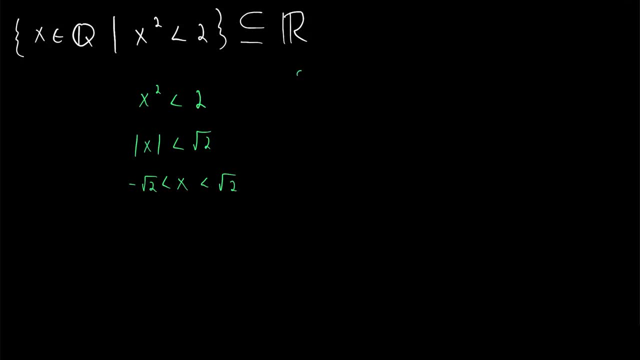 Then, since x can be any positive number less than the square root of 2, we could conclude that the supremum of our set is the square root of 2.. Similarly, since x can be any negative number greater than negative square root of 2, we may conclude that the greatest lower bound 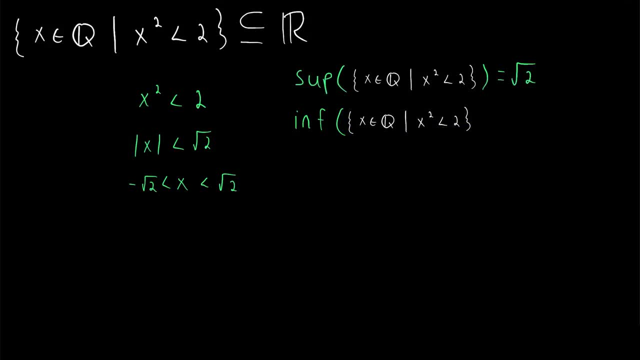 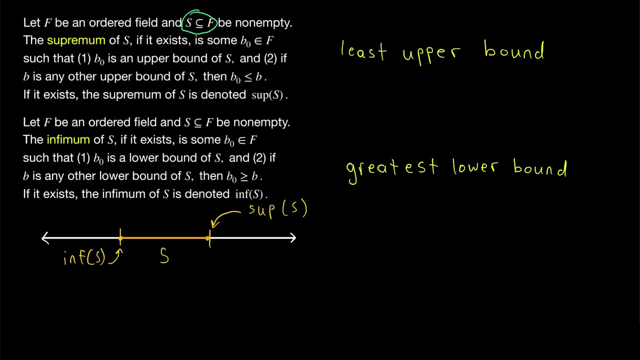 the infimum of our set is negative square root of 2.. But remember the supremum and infimum of a set have to be elements of the ordered field that we took the set from Going back to our definition. remember we take a set s from the ordered field and the supremum has to be in that ordered field. 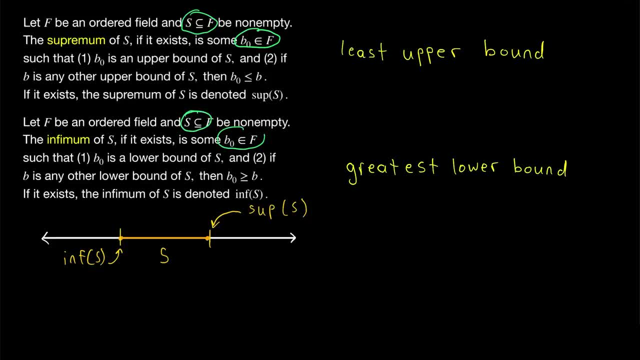 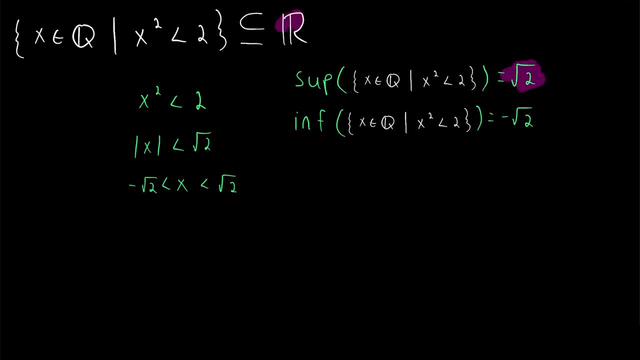 We take a set s from an ordered field, the infimum has to be in the ordered field. For our final example, this seems totally fine. Negative square root of 2 is an element of the real numbers. Negative square root of 2 is also. 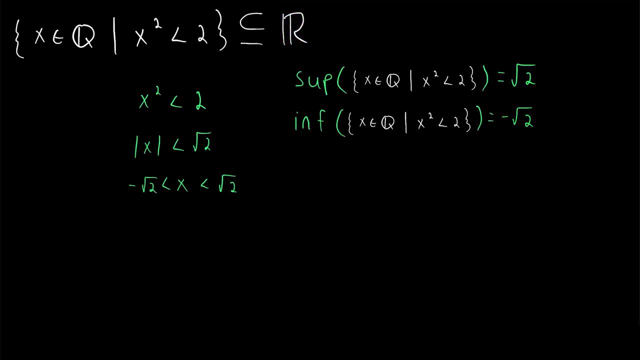 an element of the real numbers. So, then, all I want to point out is that we could have taken this set to be a subset not of the real numbers, but of the rational numbers. The rationals are also an ordered field that this is a subset of. However, in this case, the set has no supremum.